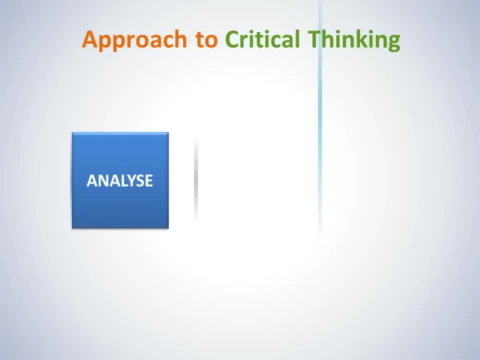 Firstly, by analysing, analyzing, asking questions of the material you're studying or researching. secondly, by making judgments or evaluations. the reason you do this is to then finally develop your own position or argument based on your readings, lectures, tutorials and extensive research. different disciplines may have different approaches to critical thinking. 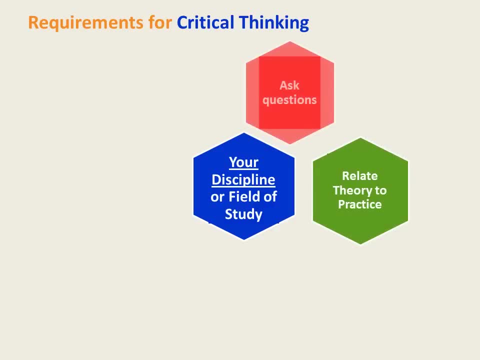 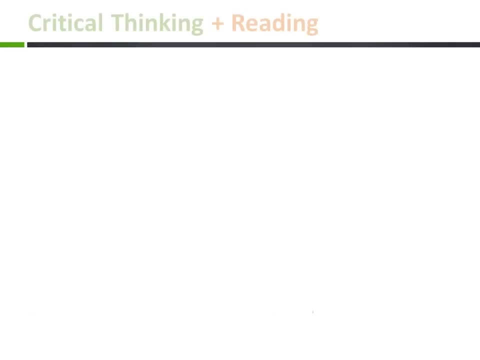 but all disciplines require you to relate theory to practice, ask questions, find and use evidence, evaluate the arguments, find links between the arguments and categorize the main lines of thinking. reading at university can be a daunting task. it's a great idea to think about the main points of a text. 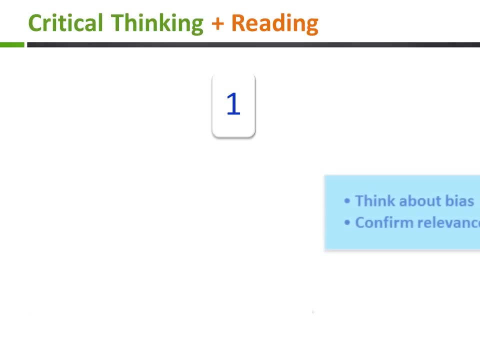 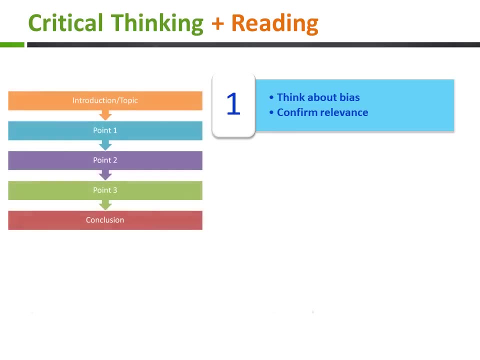 and consider how you might put them into your own words. think about bias, schools of thought or even information that you feel is missing or irrelevant. ensure you understand the stages of the argument and check that it's logical. ask yourself if the ideas presented are supported by reliable evidence. are there connections between what you? 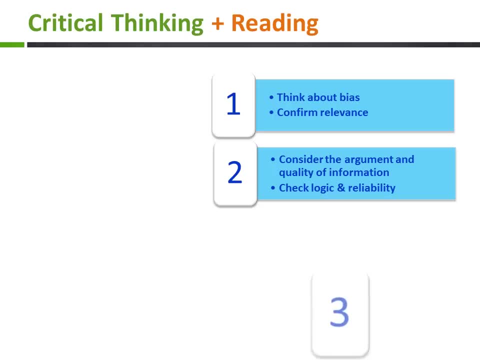 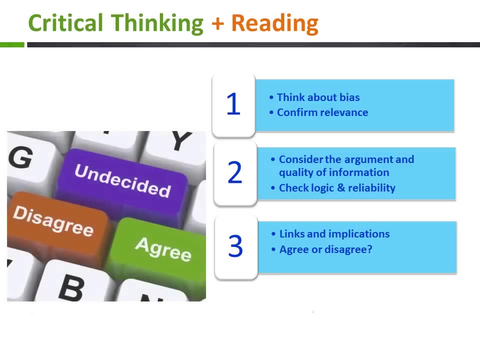 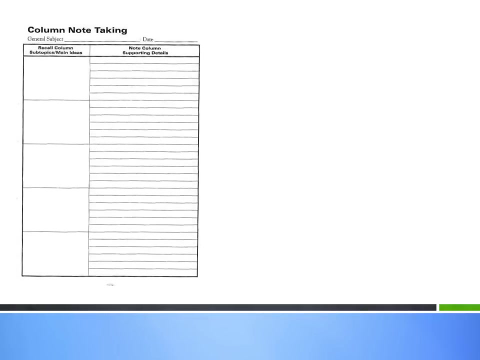 see and other texts you've read, what are the wider implications and, most importantly, state whether you agree or disagree with the arguments presented. when you take notes, divide your notepad into two columns, jot down the main ideas in the left-hand column and the supporting comments in the right-hand column. 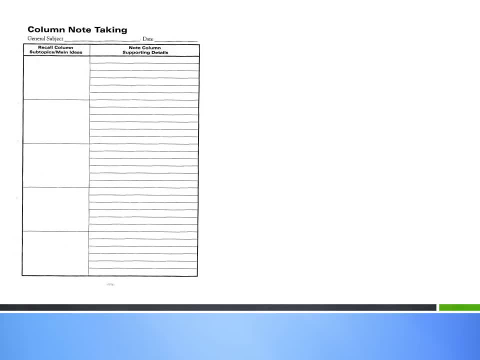 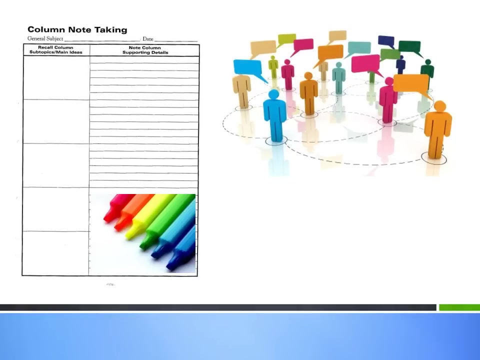 add your own comments in another color or in brackets. talk to other people about what you've read. relate and compare the text to others by looking for similar or contrasting themes. think of how you might explain what the text means to a general, educated reader. what would you have to add or subtract from the text? 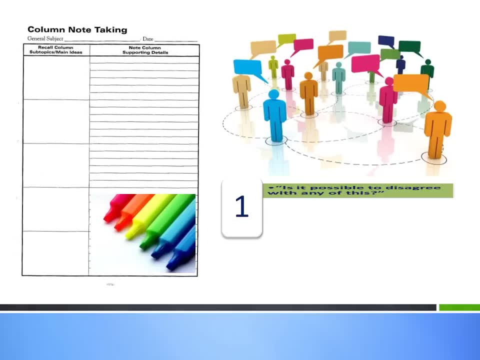 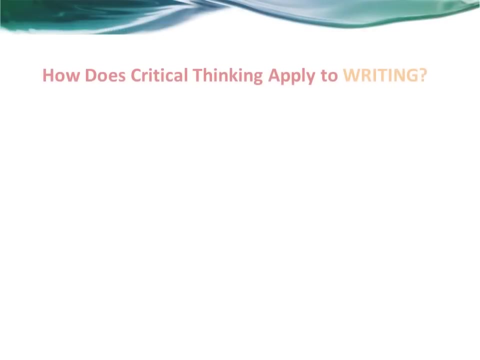 to make the argument better understood. what would you have to add to make it intelligible? think about whether it's possible to disagree with any of the arguments, and think about how you can convince your reader. critical thinking applies to writing, too, in order to improve the standard of our 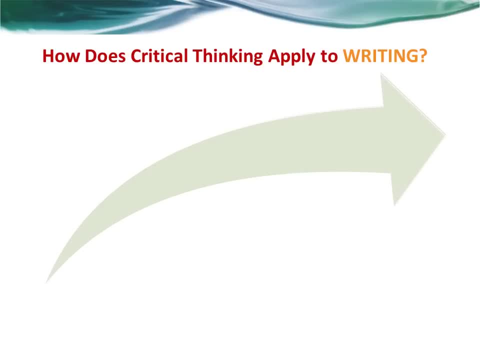 writing. we need to think about what the lecturer is looking for. we need to work out what sort of critical thinking will be involved, comparing the text with the text of the text. we need to think about what we're saying in the text. we also need to make sure that everything we say is backed up by sufficient evidence.